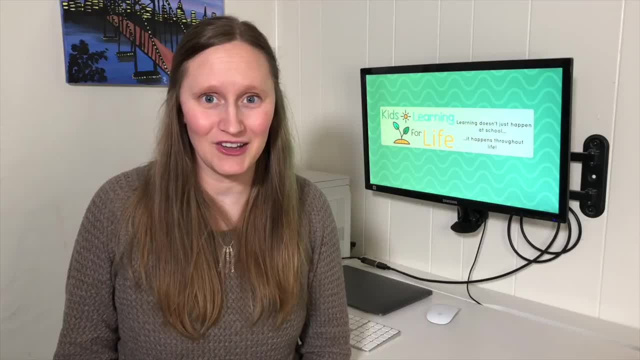 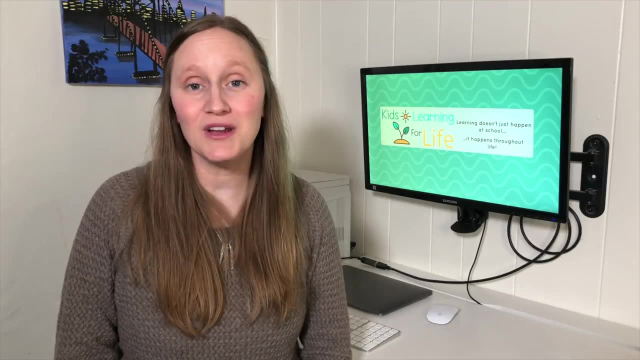 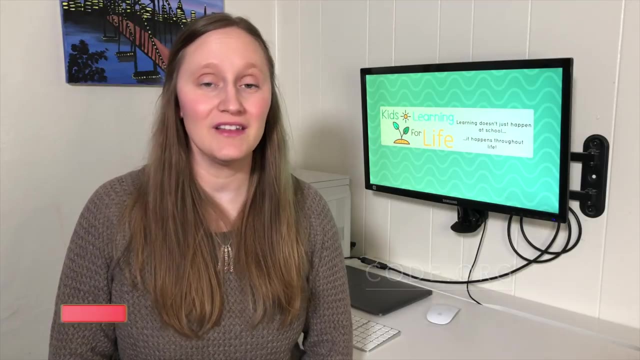 It's okay for your children to see you learning how to code right alongside them, and maybe even learning a thing or two from them. I'm going to share with you some free resources that you can use to start teaching coding to your kids today. Up first is Codeorg. Codeorg is a 100% completely 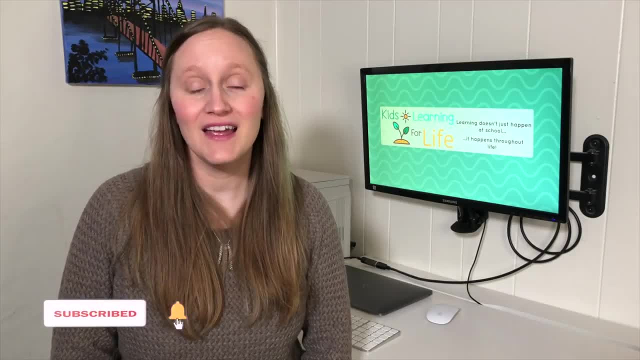 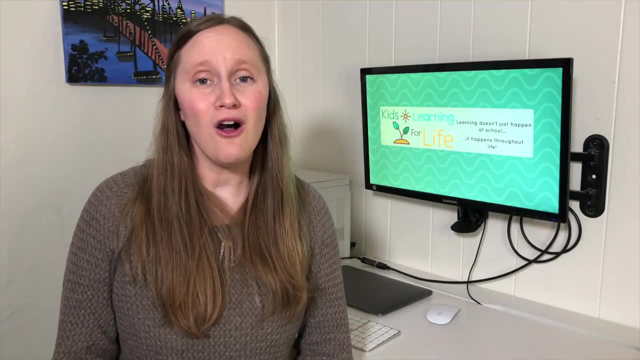 free website where students from K through 12 can go to figure out how to code. Students will create their own games, art, digital stories, all with the help of their kids. If you want to learn more about how to code, go to Codeorg. If you want to learn more about how to code, go to Kids Learning for Life and. 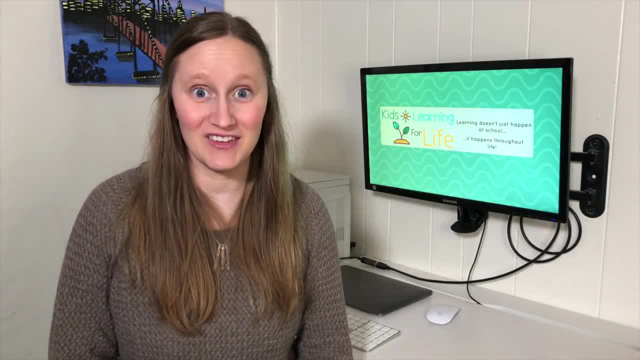 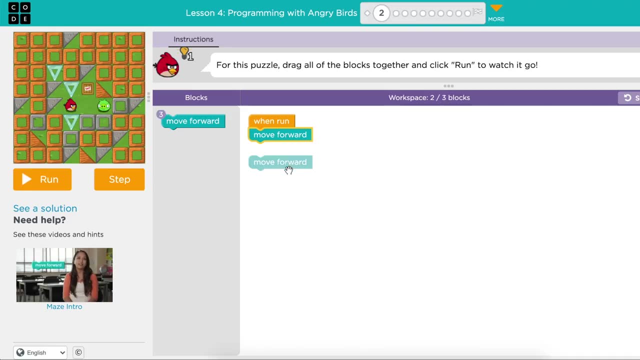 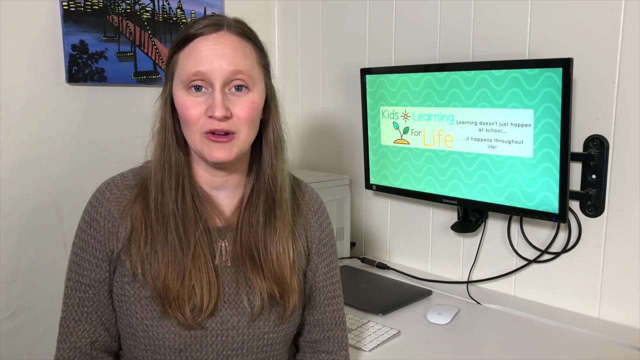 learn more about how to code. Codeorg provides lessons that are plugged and unplugged. A plugged activity just means that your student will be on the computer doing the lesson. An unplugged activity is perfect for those times where you aren't near a computer and you still want to. 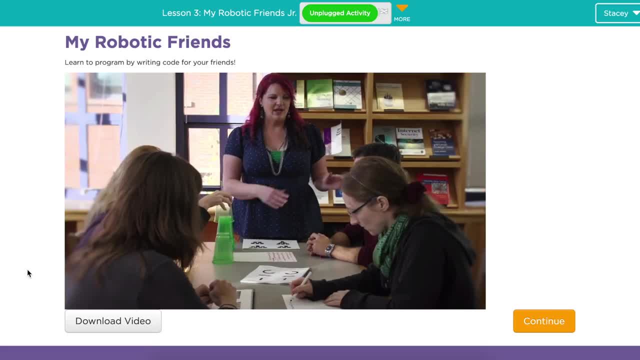 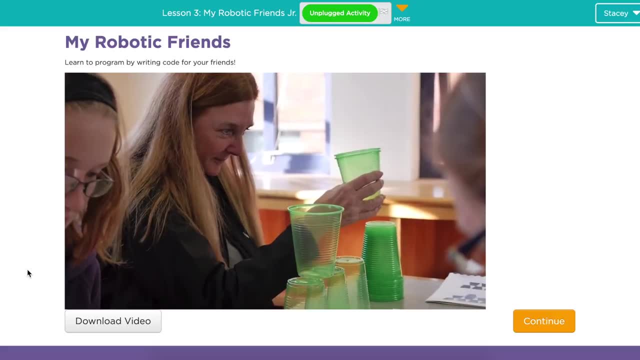 teach your kid those coding and logic skills. These unplugged activities are great for those hands-on learners that really want to see and move things around and figure it out on paper first. Then they can take those skills and apply it to the computer, Even though the 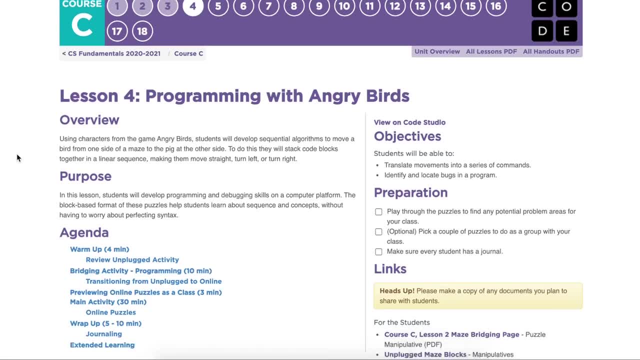 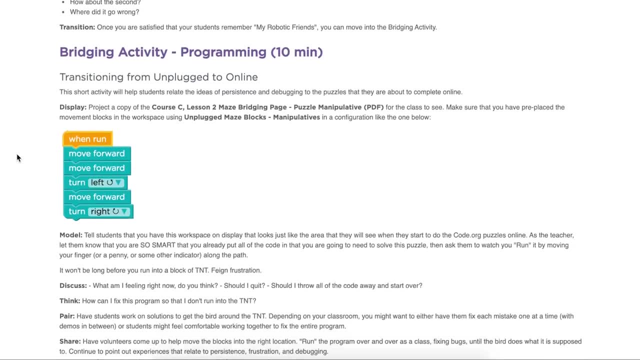 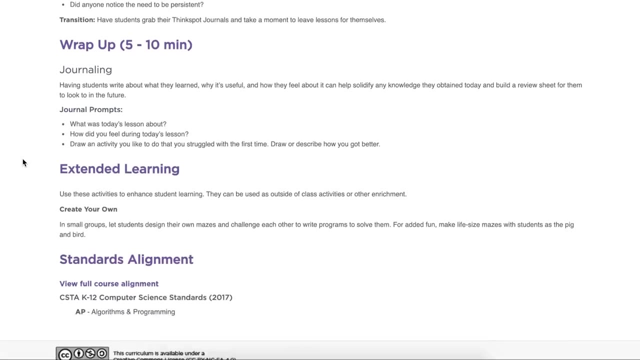 lessons are very step-by-step and student-friendly. Codeorg also includes teacher lesson plans for all of the lessons. If you don't know how to code, these lesson plans will allow you to be able to preview the material and look at everything before you teach it to your kids. 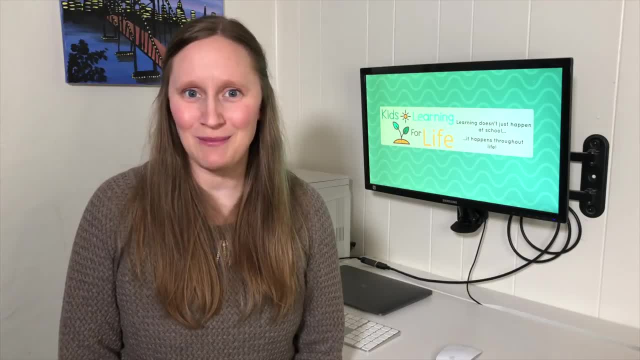 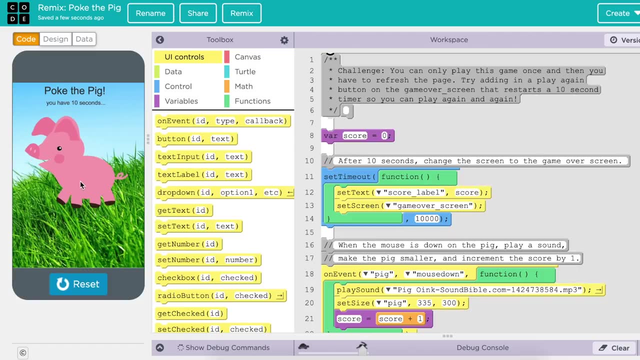 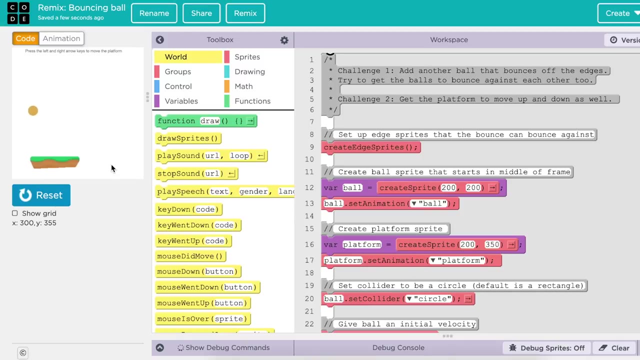 Codeorg also incorporates a few extra lab activities that students can do as well. In the App Lab, students can start to create their own app. They'll use the system interface to come up with a design and build an app that will actually work. The Game Lab allows students to go in and 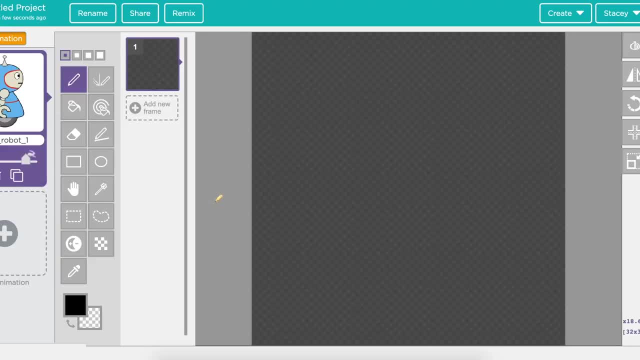 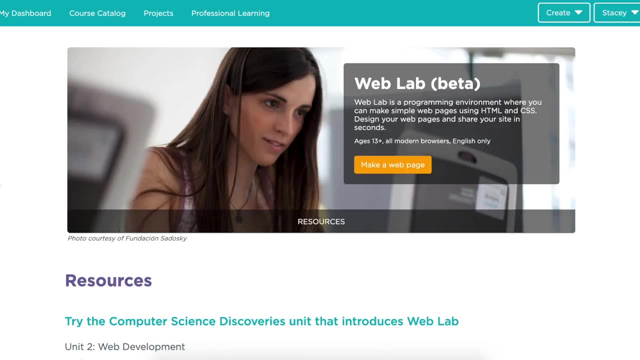 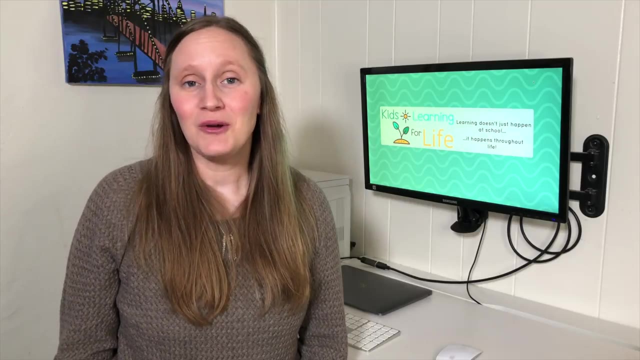 create their very own game. They can create different characters or maybe a maze and have it be actually playable online. The Web Lab is where students can start to create their very own website using code. Codeorg has also sponsored the Hour of Code event. Hour of Code can happen at: 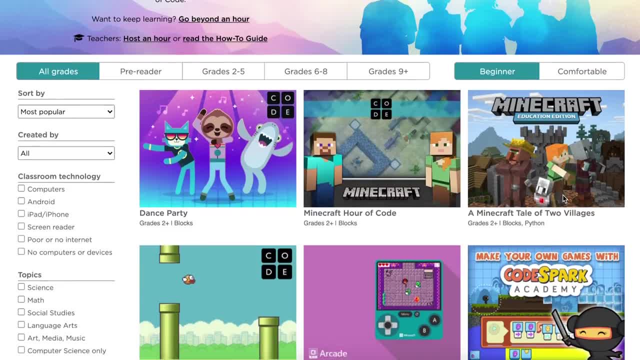 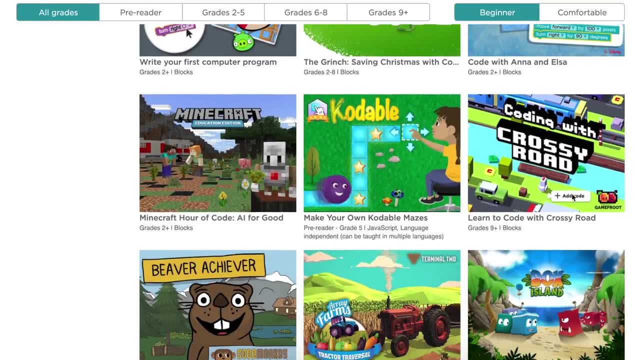 any time and anybody can create an Hour of Code activity On the Hour of Code website. you'll be able to find lots of different activities and games that children can play to extend more code learning. You can search by grade, ability level or even block versus text coding. Block coding is. 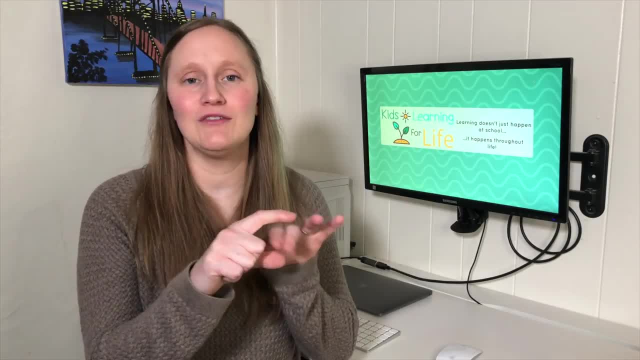 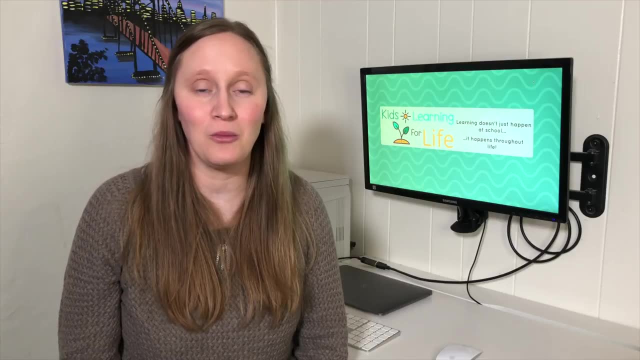 suggested for younger users because it has all of the words inside of a block and you can connect the blocks together to create your code, While text coding is recommended for older users that already know how to spell words and type on a keyboard because they're going to be typing. 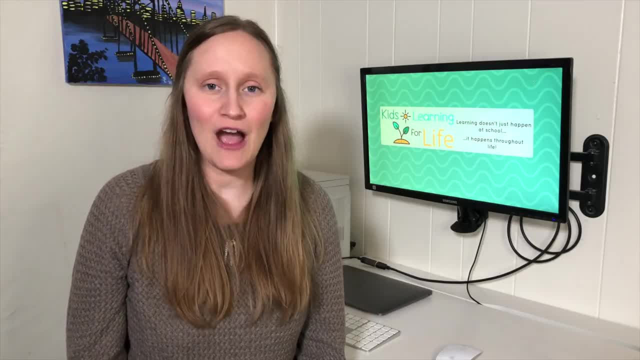 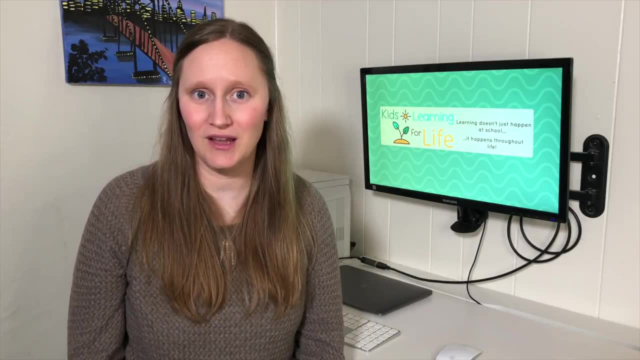 out their code in full form. I would best recommend the Hour of Code app. if your kids are really seeming to pick up code and you're looking into maybe another paid version of coding, This could be a great place to look at some of those other third-party vendors. There are lots of other. 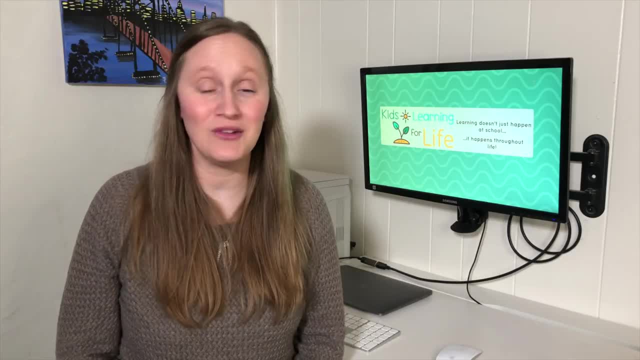 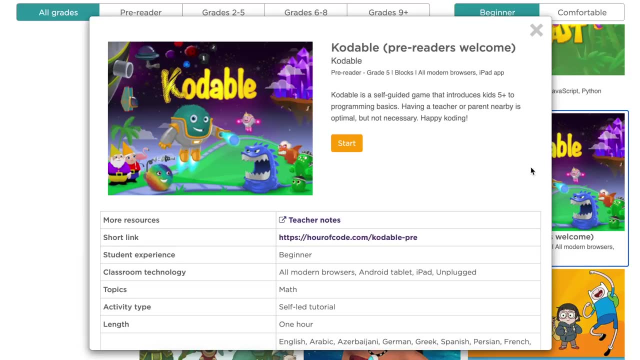 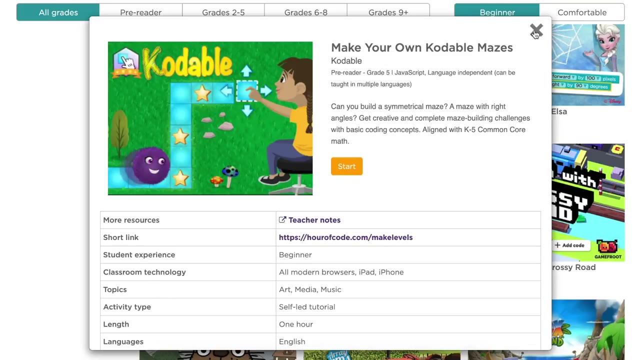 paid coding platforms out there that you can try out, such as Code Monkey, Codable Tinker and Codakid, just to name a few, And each of these companies have created a little Hour of Code. So think of it as a sample, So you can try out some of the activities there to see which program your kid 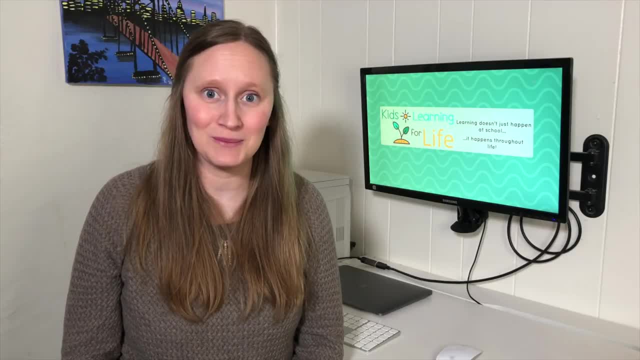 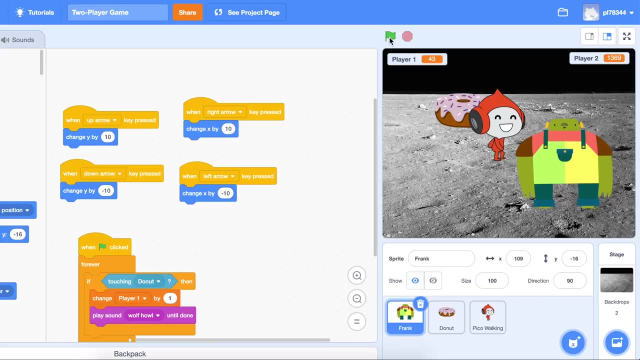 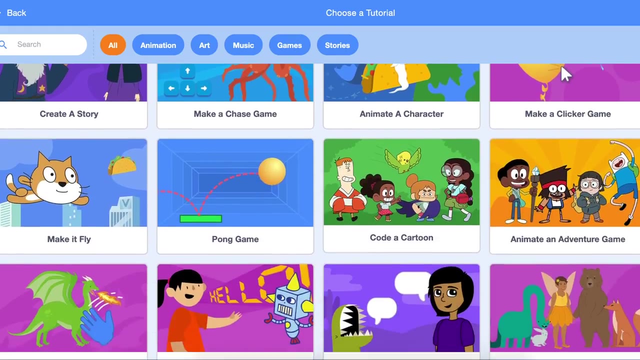 might like best before you have to go and buy something, if you choose. The next program I want to mention is Scratch. Scratch is a simple block coding website that allows students to create simple images, stories, games and more. all on the website. Scratch has tutorials right on their 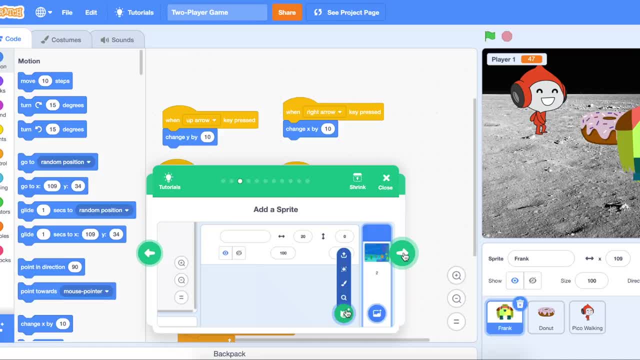 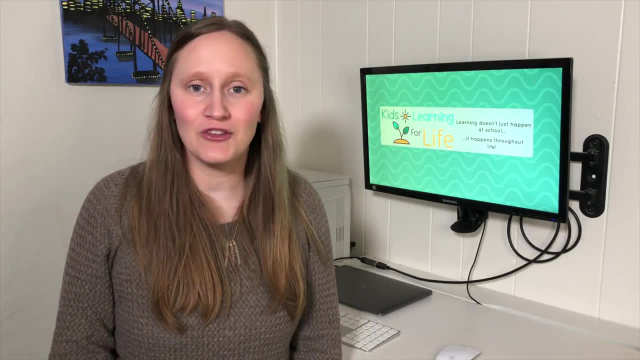 website that will help teach you, step by step, how to do some of the different activities. Remember, with coding you really can do almost anything, So really let your children use their imagination and create anything they can put their mind to. For younger coders, you can use Scratch. 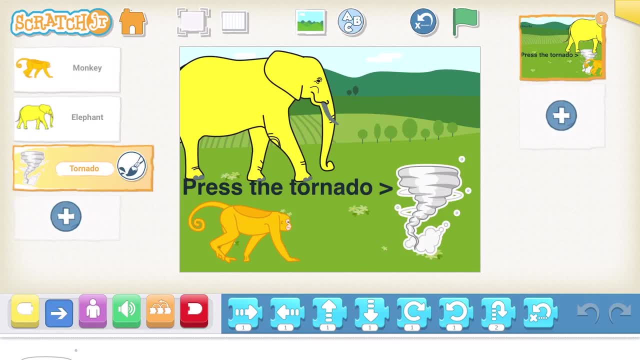 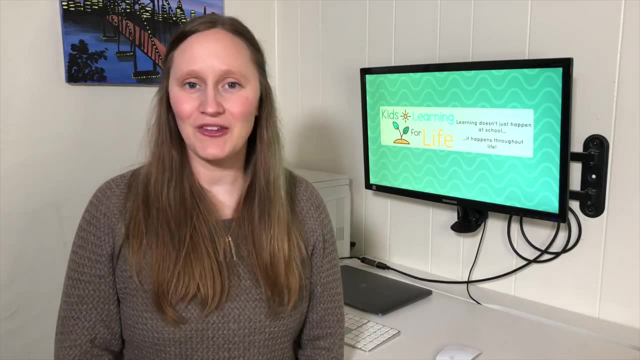 Junior, and this is available on the iPad. Scratch Junior uses the simple block approach, but in this version they're using images rather than actual words. Scratch Junior also has tutorials in their app that'll teach you how to do some fun things. If you'd rather be able to have the Scratch Junior. 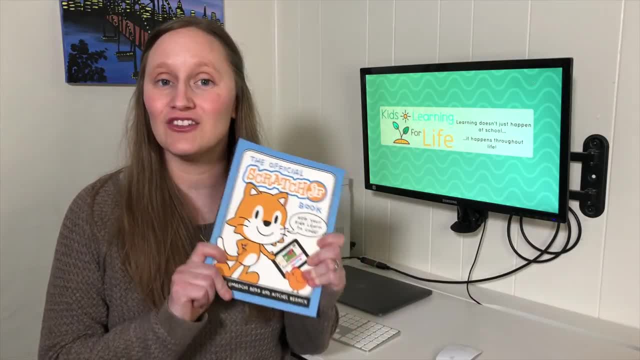 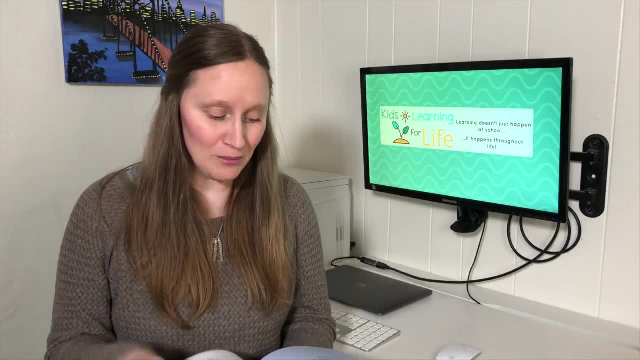 tutorials more tangible. you can go to Scratch Juniorcom and search for Scratch Junior tutorials. Then you can try the Scratch Junior tutorial book. This basically has all the same tutorials but in a print form, so you can just simply open it up and be able to walk your child through what they're. 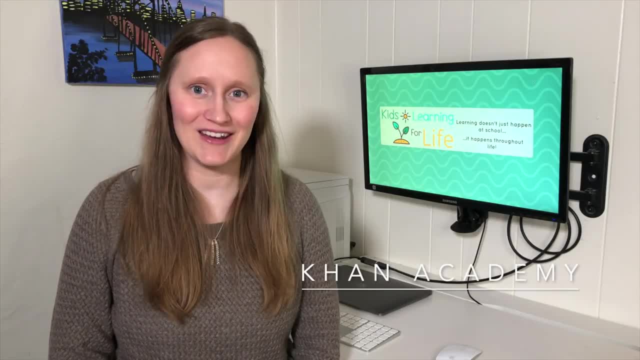 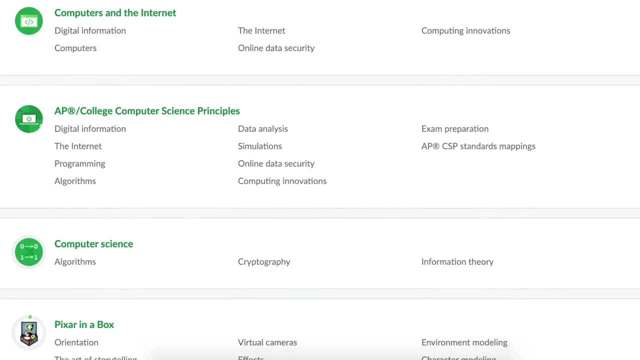 trying to figure out. The next resource I want to recommend is Khan Academy. Khan Academy has a couple different computer science programs. They have computer science, computer programming, computers in the internet and Pixar in a box. The first three are going to walk you through some of 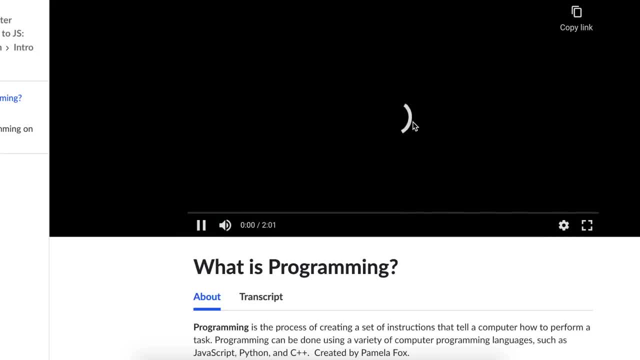 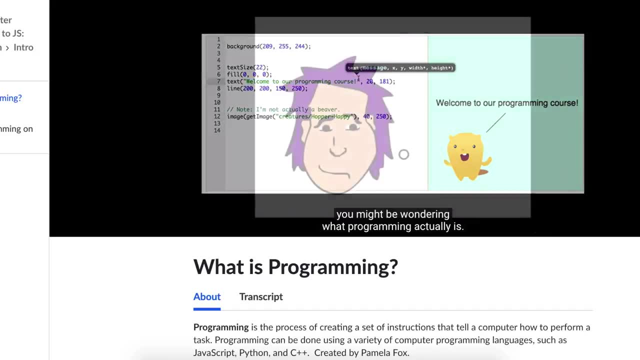 the computer science, the internet and even some programming. The step-by-step lessons have videos embedded and even some text that you're able to read through and follow along in their program. The Khan Academy program is self-paced, so students can pick and choose how much they. 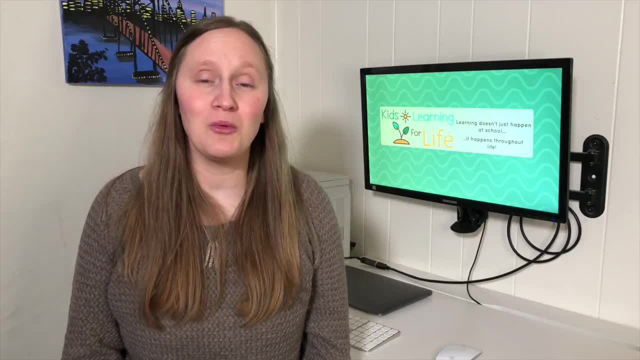 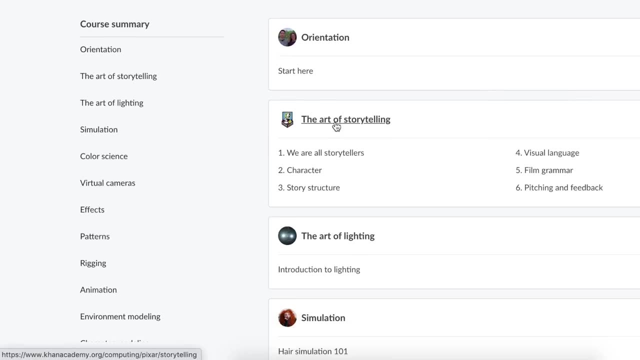 want to do each day. The Pixar in a box program goes over what it takes to create computer animation. If you have a young animator in your life and they are interested in maybe becoming a computer animator, this is a great place to start and just kind of let them see what they're going to do. 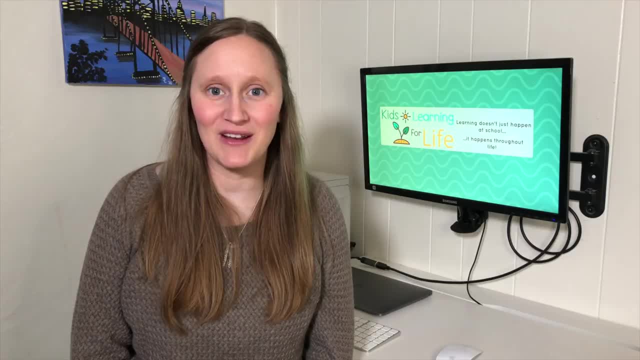 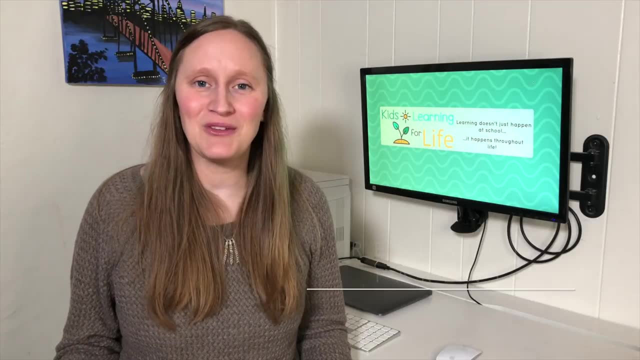 What it takes to be a computer animator and what skills they're going to need. The last resource I want to recommend is going to be a completely computer free option. I found this free resource on the Research Parent blog and they offer a free printable that allows you to take coding from the. 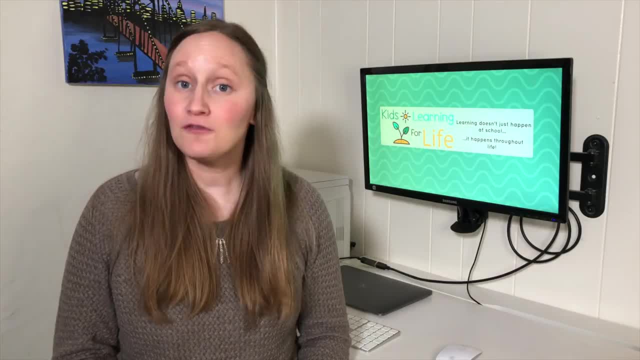 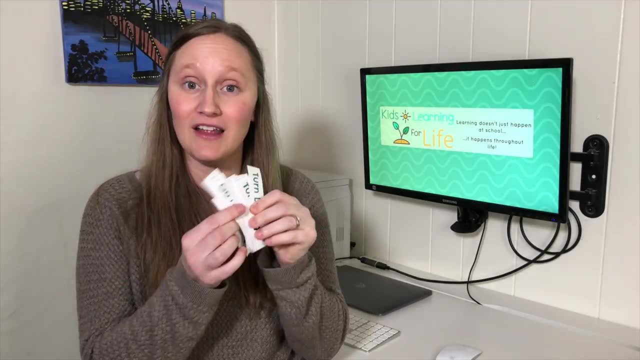 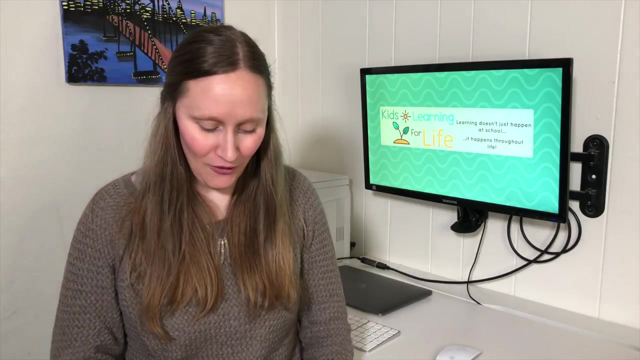 computer and puts it into something tangible that you can hold. The free printable includes all sorts of little cards that you're going to have to cut out, but like turn left and go forward and turn right- Oh, that's still go forward. There's a turn right in here somewhere. There it is, and what you can do is it will also give you. 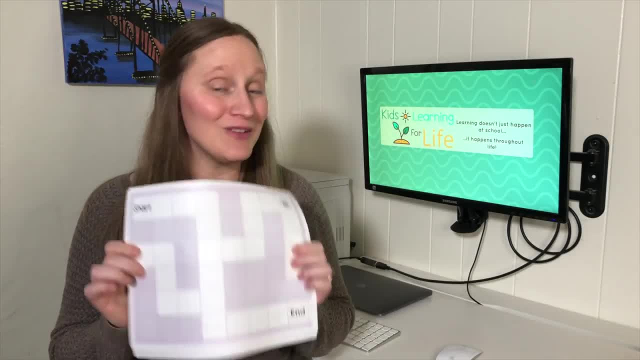 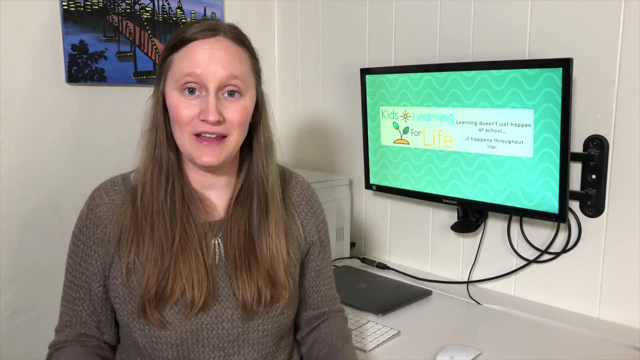 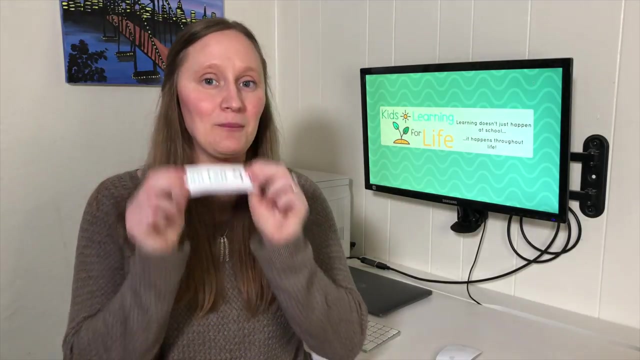 different mazes, and so it's intended to work with Legos- either Duplo or the regular size Legos- and you lay the mat out, build your little Lego maze around it, and then your children will be creating the code using basically block coding, but in paper form. So this is kind of similar to. 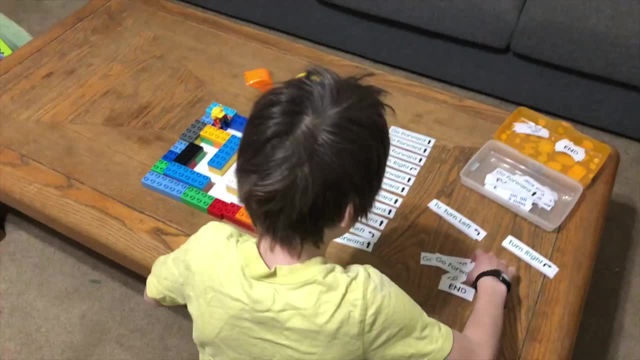 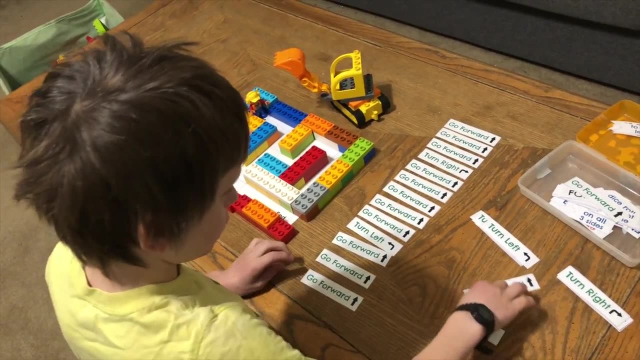 maybe an unplugged activity that codeorg would have. but here it's a free printable that you can cut out, and you could even laminate them. I just don't have a laminator so I have not done that yet, but you can laminate them so that your kids can create their own mazes. 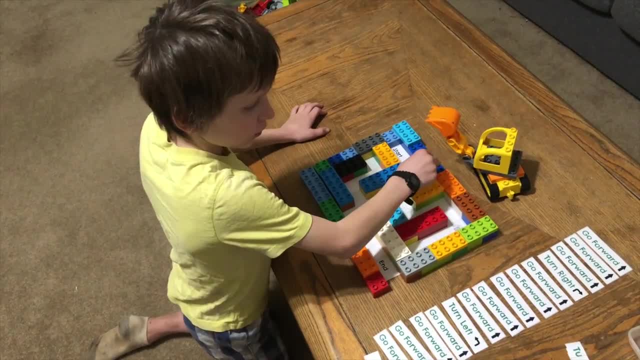 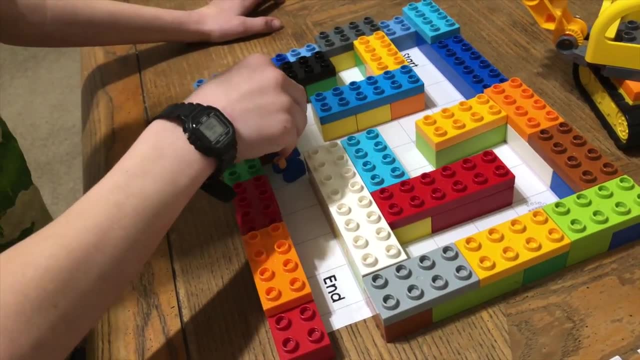 and use this to guide a little character, so that you can come over and they create the code and then you can run it through for them and say, hey, let's see if this works and see if you can get the little character from the start all the way to the end. My kids had a lot of fun with. 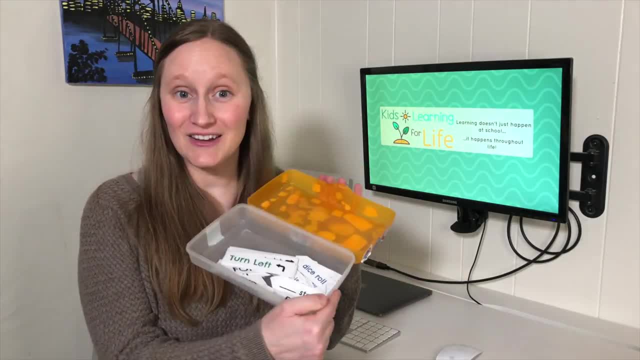 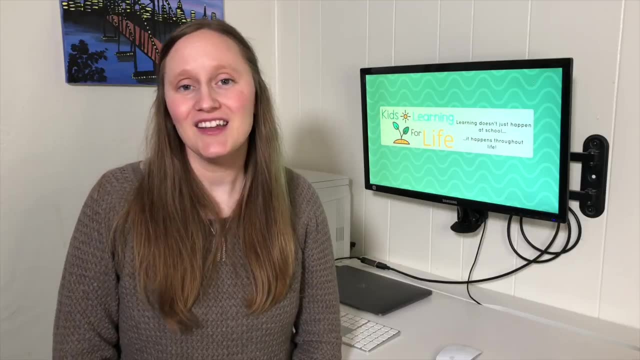 this activity, and I'm definitely going to be keeping all of these in a little container so you can use them in the future. There you have it: some free resources that you can start using today to start learning and teaching your children how to code. Coding doesn't have to be scary and